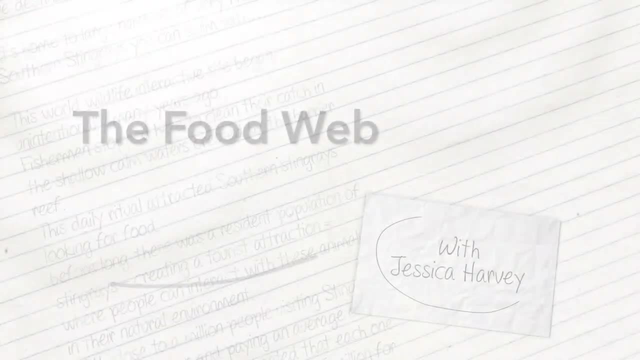 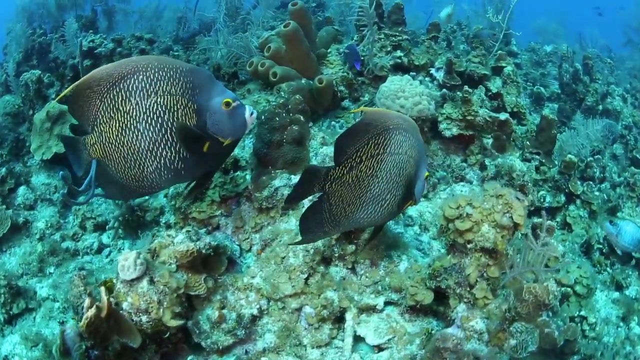 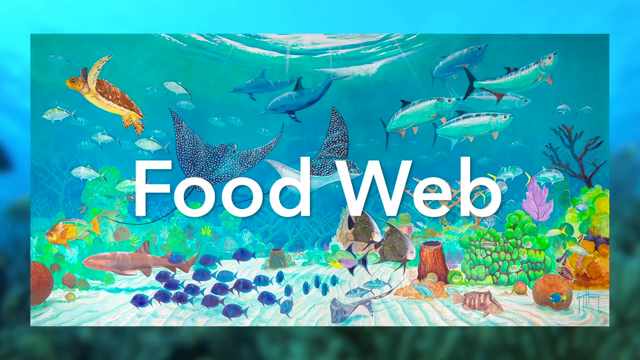 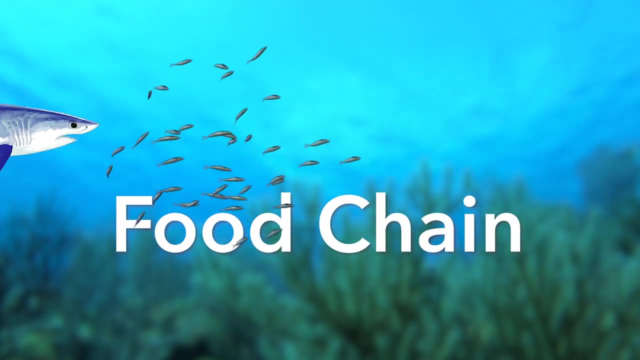 At the surface, the ocean seems simple, but dive in and you'll find a complex ecosystem that needs to stay in perfect balance. A food web is how living organisms interact and depend on each other to survive. A food chain is the order in which living organisms are consumed. For instance, the big fish eats. 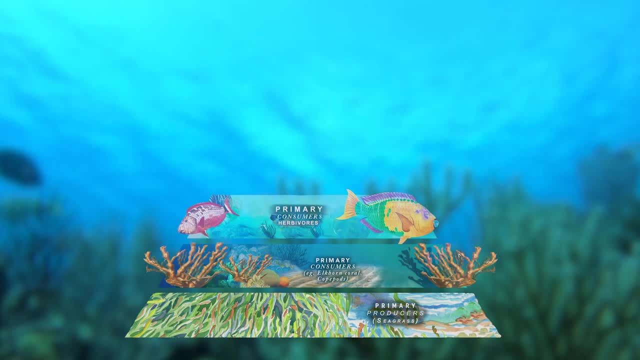 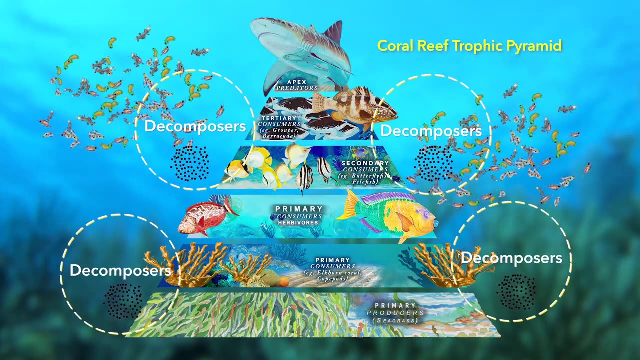 the little fish. For the next few minutes, we're going to look at how everything is connected through a coral reef trophic pyramid. Here's how it works. At the bottom you'll find the primary producers, in this case seagrass, which. 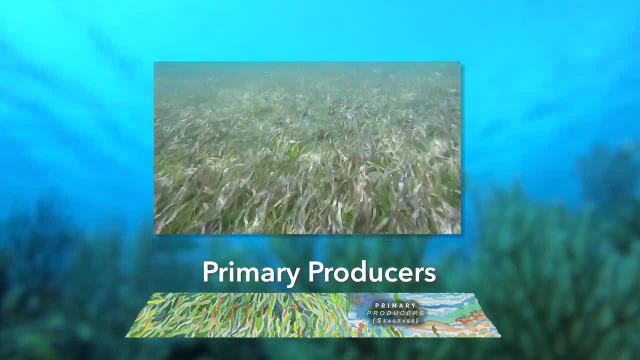 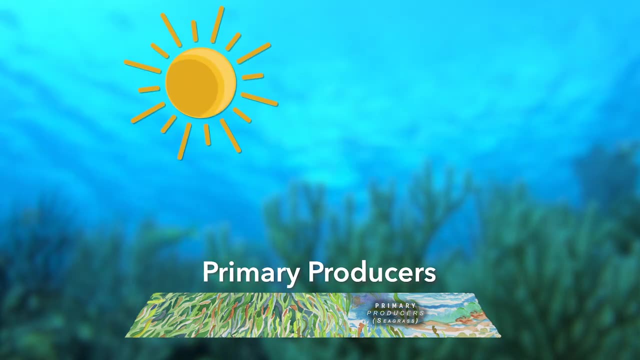 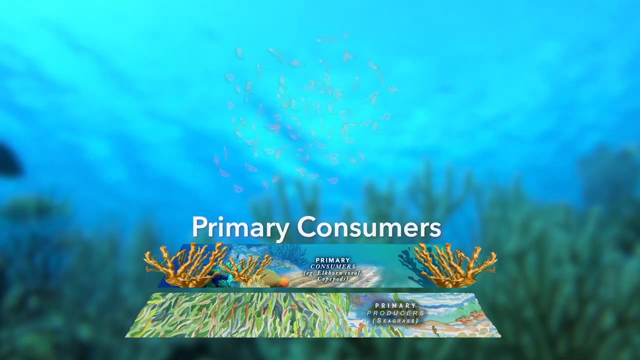 uses the sun's energy to produce food through photosynthesis. These primary producers are the foundation of the food web and the beginning of our pyramid. They can produce their own food from the sun. Above this level are the primary consumers: microscopic animals such as. 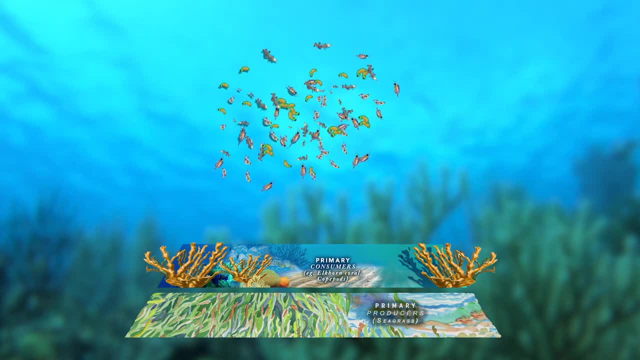 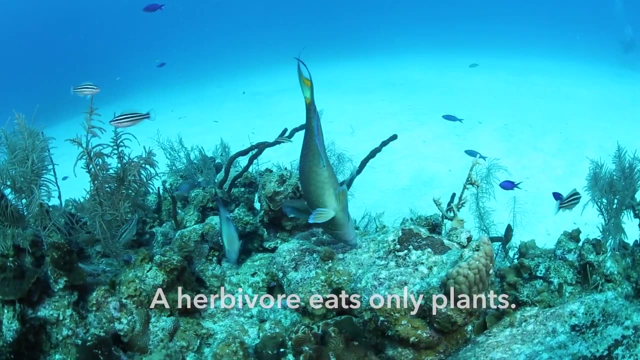 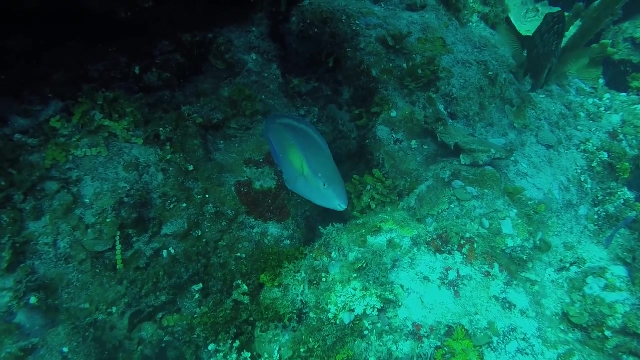 corals and zooplankton that feed on all the primary producers. You can also find herbivores at this level. Herbivores are animals that eat only plants. For our example, we show parrotfish. Parrotfish are critical to a reef because they 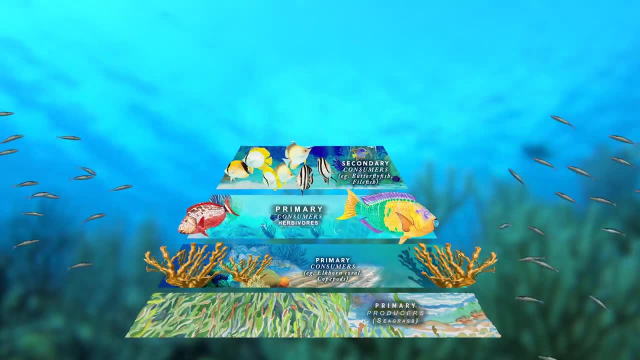 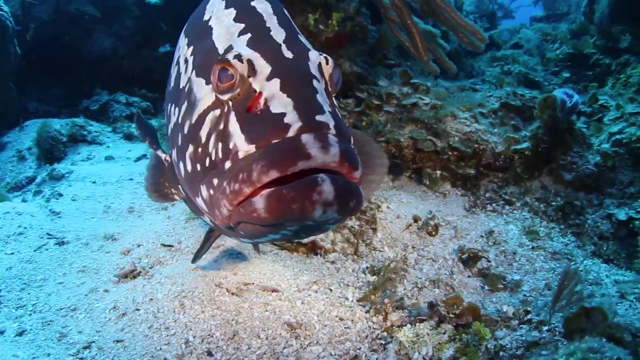 only eat algae. Next we move to the secondary consumers, mostly carnivores feeding on primary consumers, or the herbivores. A carnivore eats other animals. Above the secondary consumer level, we have the tertiary consumers: medium reef predators such as groupers and barracuda, feeding on smaller fish At 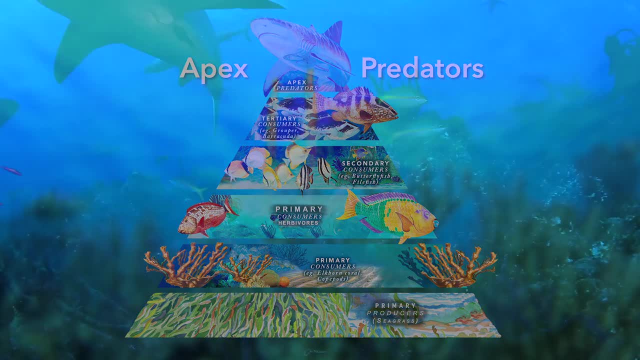 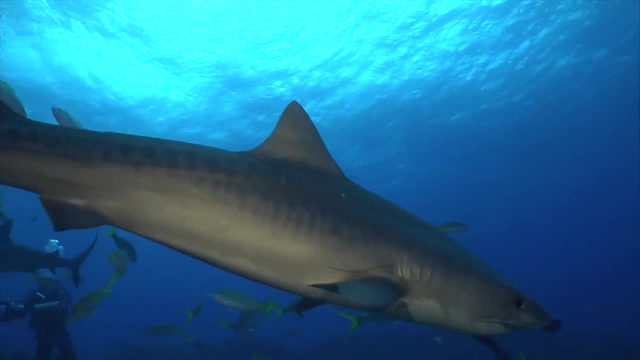 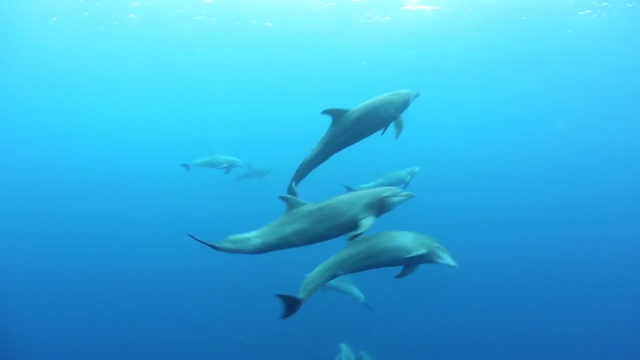 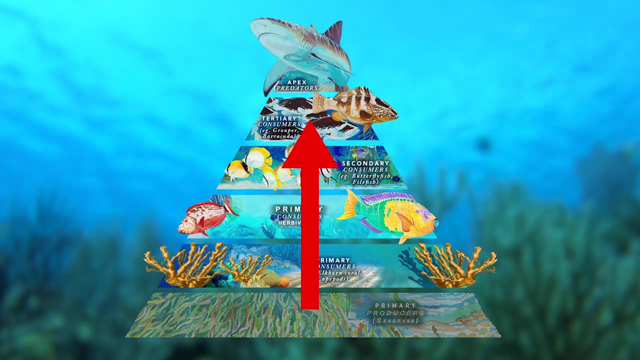 the top of the food web are the apex predators. In this example, sharks hunt and consume the medium reef predators. Sharks also keep the ecosystem clean by eating other animals. You can also find marine mammals at this level. Notice how the levels get smaller as you move up the pyramid. When animals feed, energy is.